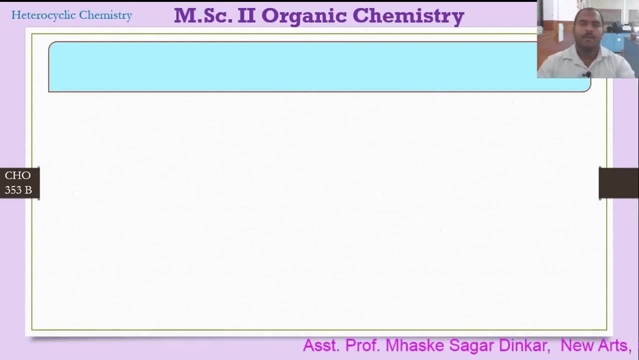 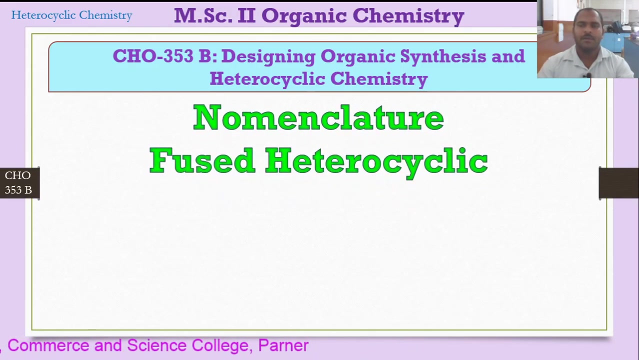 Good morning friends. In previous lectures we have seen a heterocyclic nomenclature for a monocyclic system. Now in this lecture we are going to continue with our CHO3PPTB heterocyclic chemistry and we are going to see a nomenclature for a fused heterocyclic system. 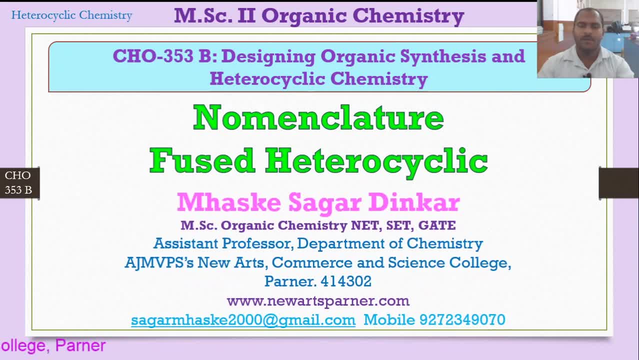 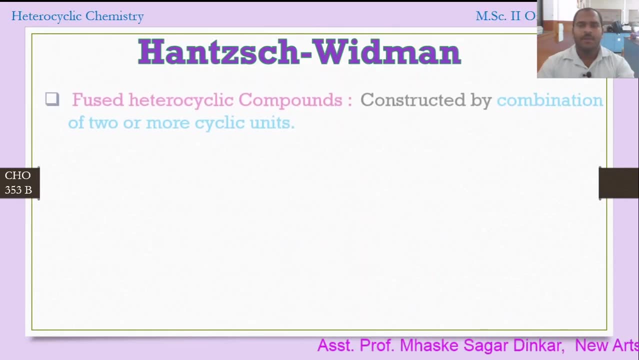 So, with the help of Hans Widemann rules, we are going to go for the nomenclature of the fused heterocyclic system. So let's start our discussion with a fused heterocyclic system. Here we are considering a fused heterocyclic system for a nomenclature. 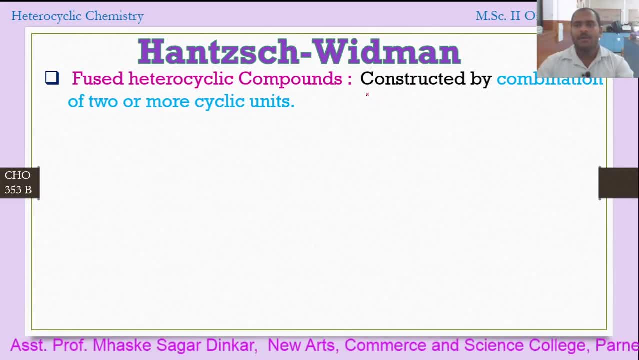 What are the fused heterocyclic compounds? These compounds are constructed by a combination of two or more cyclic units. When two or more cyclic units are joined together, they are called as a fused compound, And when there is a presence of a heteroatom in a cycle, it is a fused heterocyclic compound. 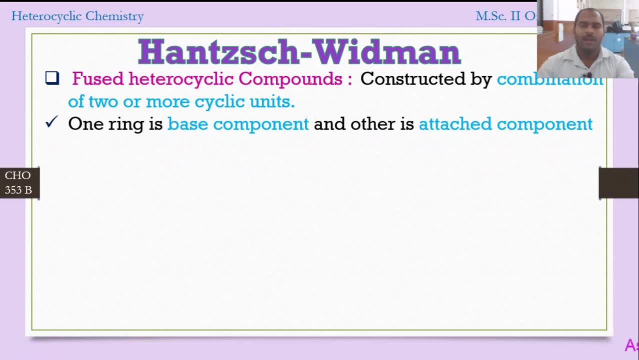 In a fused heterocyclic compound one ring is a base component and another ring is an attached component. So we are considering a fused heterocyclic system. So we are considering that in a fused heterocyclic one is a base component and other is an attached component. 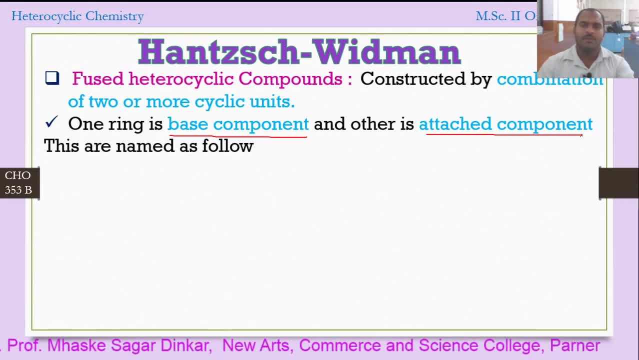 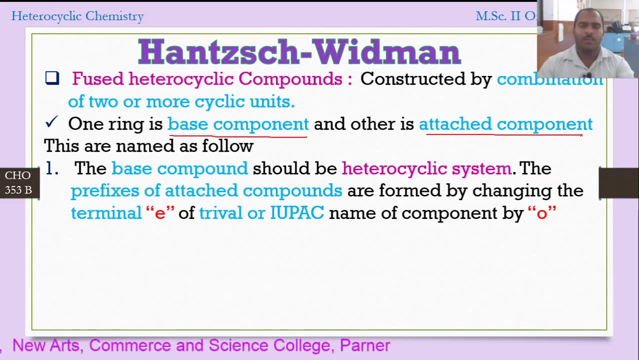 These are named as follows. So there are certain rules for naming of these base components and attached components. Let's consider rules one by one. The base component should be a heterocyclic system. That is an important thing to remember. That is a heterocyclic system in a fused system is a base component. 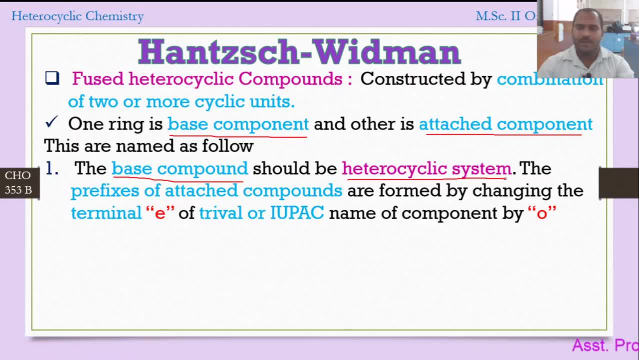 The prefixes of attached compounds are formed by changing the terminal E of triangle or the IUPAC name of a compound by O. So in this case, what we are considering, the attached component prefixes are, having certain modification, The terminal E of that attached component, IUPAC. 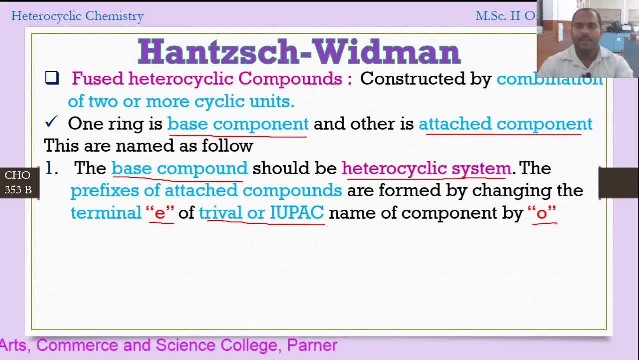 So the attached component, either triangle or IUPAC name, is replaced by O. Let's consider some examples Here. we can see: Suppose, if a pyresine is attached component, then pyresone, that is E of pyresine, is replaced by O. 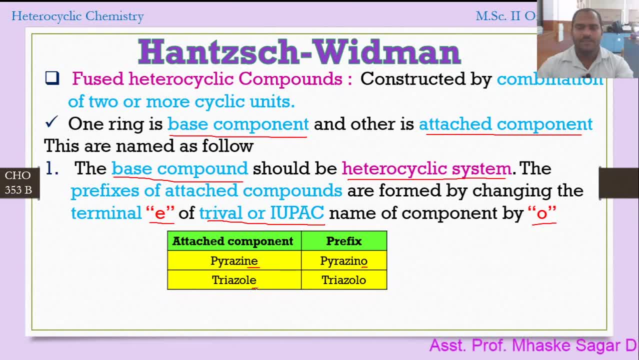 Okay, So here triazole is attached component, then triazolo will be the prefix for this. For first rule we have to understand that base component is a heterocyclic system and attached component, terminal E of triangle or IUPAC name is replaced by a component O. 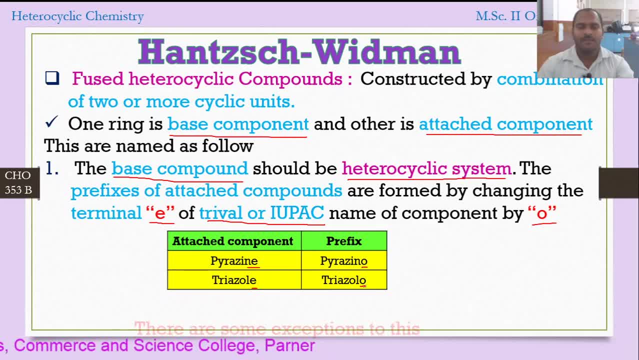 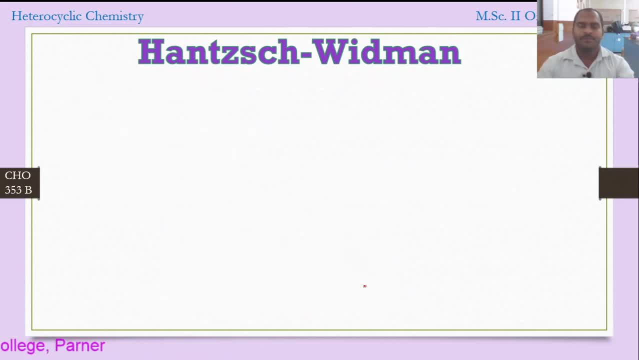 Okay, So here we have taken two examples, But for this rule there are certain exceptions also that we are going to see in the examples. Okay, So let's go for the next. Location of fused system. Location of fused ring. 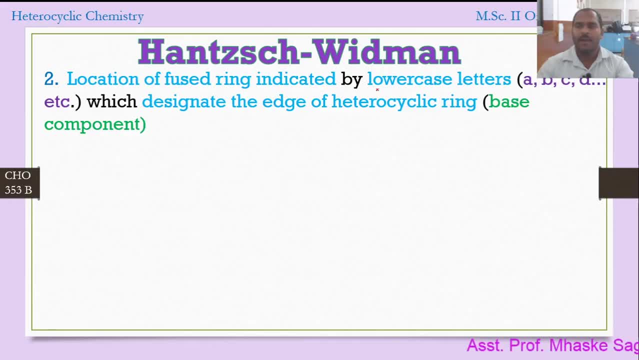 Location of fused ring is indicated by lowercase letters, that is, A, B, C, D, etc. which designate the age of heterocyclic ring. that is the base component. Okay, So what is this second rule suggests? 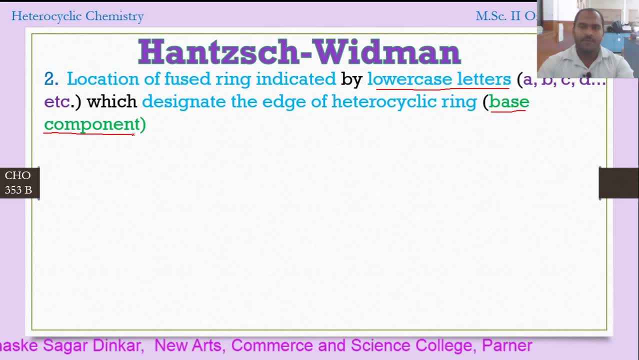 Second rule suggests that for location of a fused ring system we have to indicate this location or joining With the help of lowercase letters, either A, B, C, D, etc. that can be used, which designate or suggest which age of the heterocyclic ring is going to be attached with the attached component, or which age is there for the formation of a fused heterocyclic. 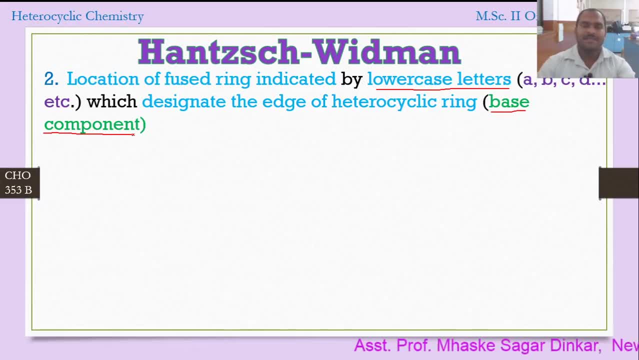 Okay, So let's understand this second rule in detail with the help of an example. Okay, Now consider these two rings. Okay, So let's understand this second rule in detail with the help of an example. Okay, Now consider these two rings. 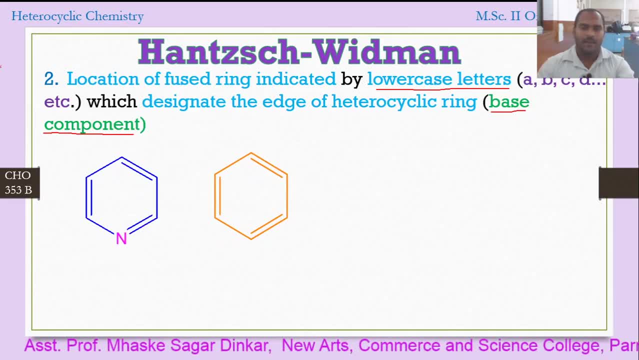 Okay, Here what we are considering. we are considering that the first ring, the first ring, Here there is a heteroatom, I told you, and second is a benzene. Now, you can see here, as there is a heteroatom in this ring and it is a cyclic system of 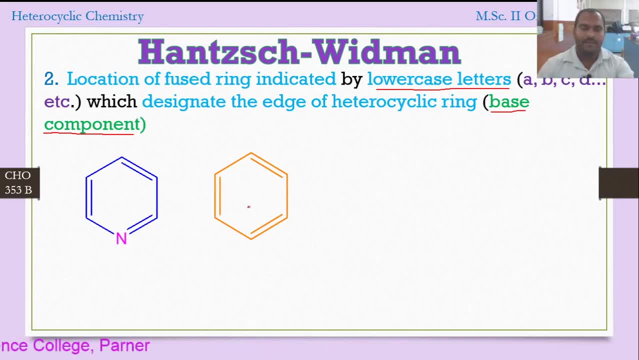 and only carbocyclic, no heteroatom. So we can say that the first one is a base component which is a pyridine Right. second one is the attached component, which is a benzo. so here we can consider: e is replaced by: 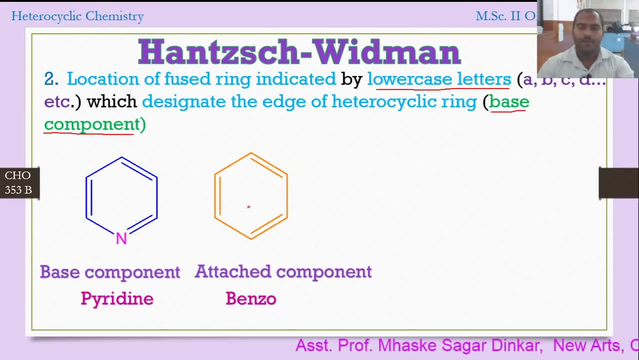 o, it is an exception for this. okay, so let's see how, if they combine, what will be the name of the compound and how we can designate the name of the compound. so for joining up with these two, we can have a different edges, okay, so let's consider how. 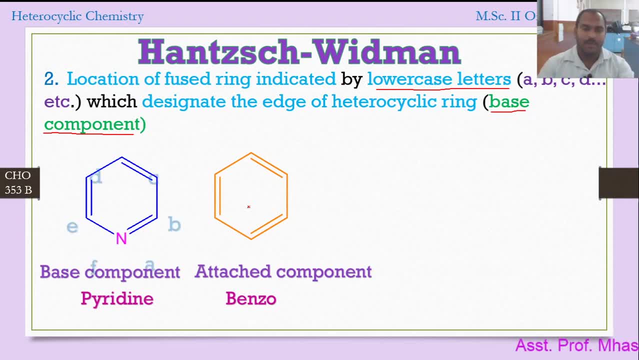 we can denote or edges for the base component. here we are denoting the edges for the base component, a, b, c, d, e, f. i have gone in this direction. you can go other directions okay, but for shape of a news i have written like this: now let's consider the one compound which is for my 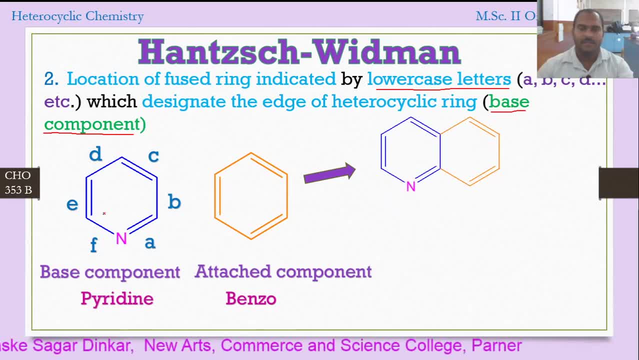 combination of these two. that is the fuel system. now, here you can see these two are fueled and use the formation of this compound. now we have to give the name of this compound and find out what is the age for the attachment. so age is denoted by the lower cage. so here we are, denoting by the lower case and try to make 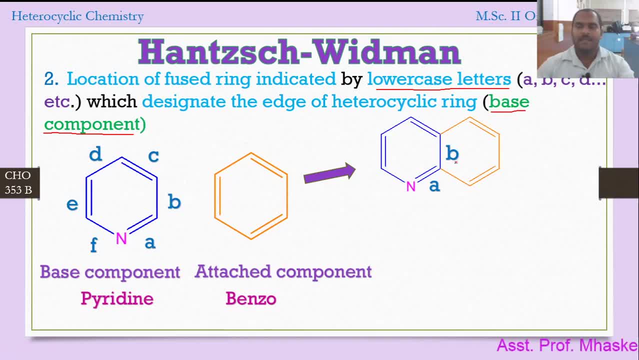 having a possible lower cage later. that is a, b. okay, so b side of this ring base component is attached with this attached component. so let's see what will be the name. so name will be benzo. it is attached component, so brings. so you will convert. in square bracket we are writing the b. 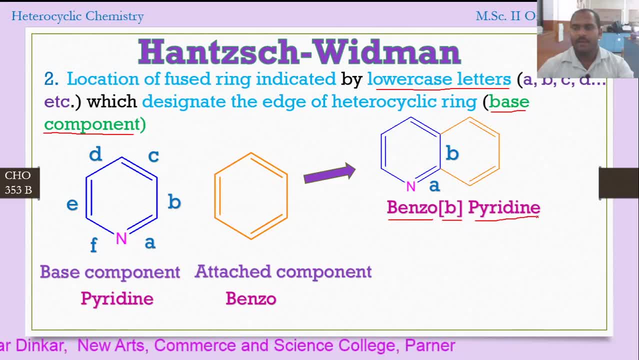 which indicates the age, and pylene is the name of the compound. so here we are having a name of the compound: benzo, square bracket b, pylene. what it indicates? it indicates that benzo is an attached component in square bracket b, indicate that b is the site or h at which we are having a fusion. and 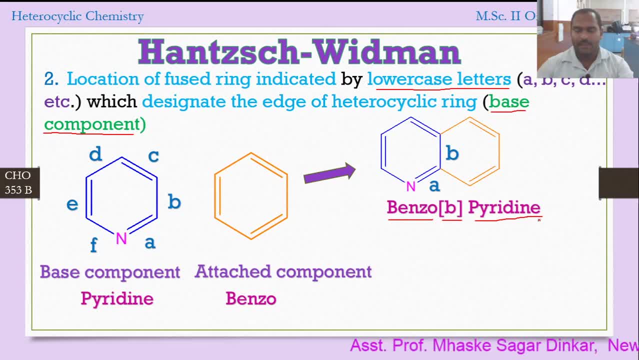 the base component for this. now let's go for the same compound, same type of the fusion, but slightly the different age. now you can see here there is a difference. here we are having a nitrogen closely attached, here we are having one carbon in between them. so we are having the ages a, b. 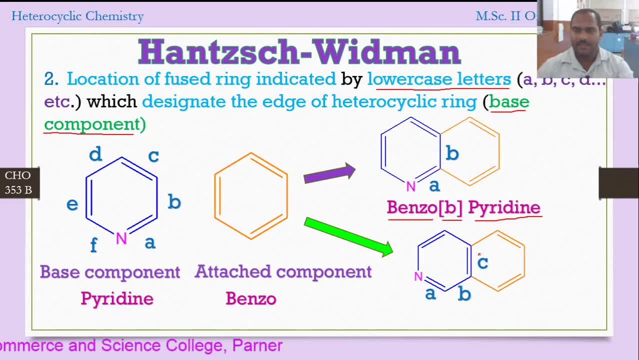 and c: a, b and c. now what is the attached? a attached is a, c. so if name of the compound will be benzo c- pyridine, okay, why benzo c, pyridine, benzo c and pyridine benzo is the attached component. 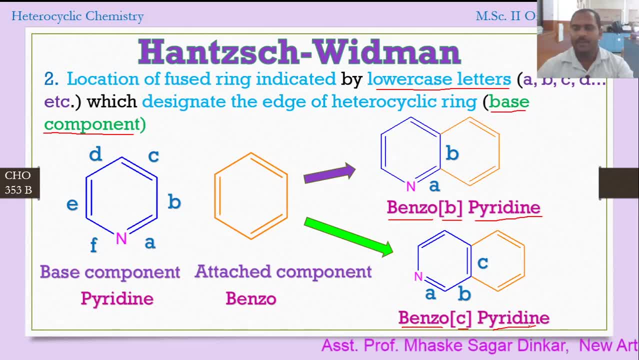 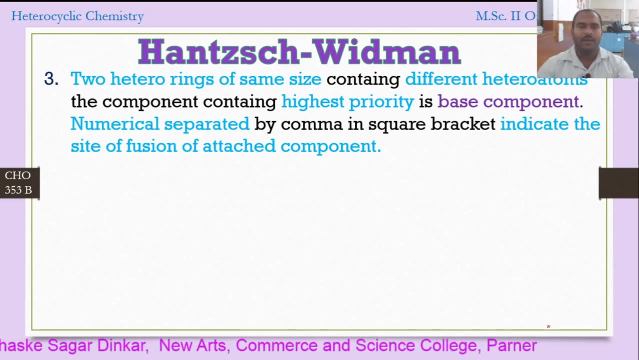 c is the site where we are having a future, and pyridine is the name of the compound. so in this way we are having the name of the compound. so let's move further. for the next rule: two hetero rings of same size containing different hetero atoms. 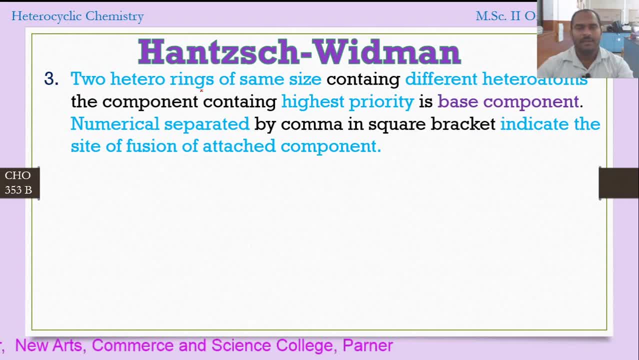 suppose if this is the case, that is, the two hetero rings of same size containing a different hetero atom, the component containing the highest priority is a base component. okay, when we are considering a huge heterocyclic system and in that huge heterocyclic system, if both the rings are. 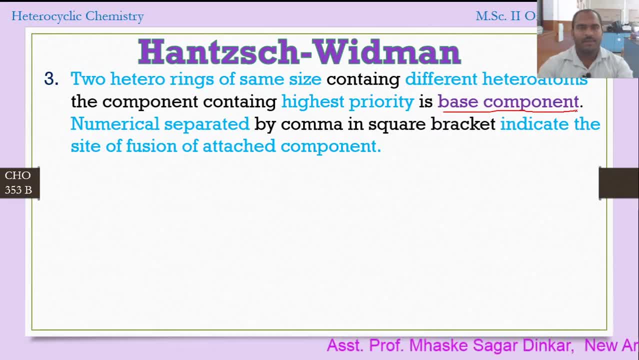 containing the hetero atom. they are often same size but different hetero atoms. in that case the highest priority atom will have a base component. okay, so the hetero atom which is having highest priority that cycle is considered as a base component. the numerical separated by comma in square bracket indicate: 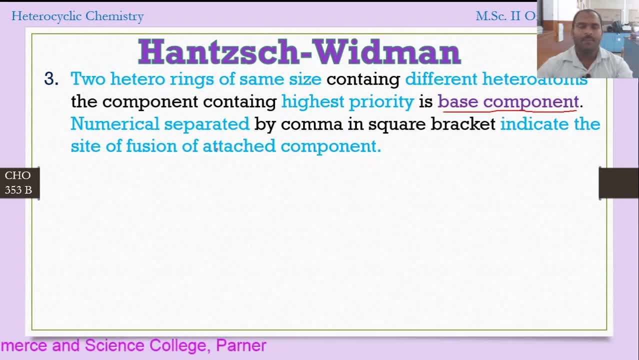 the site of fusion of attached component. okay, so in that case when we are writing the name in name, we are writing it in the square bracket a, certain numbers. that number indicate the site of fusion of the attached component. okay, now, up till in base component we have seen a site of fusion where a, b, c- these are the sites for attached component. 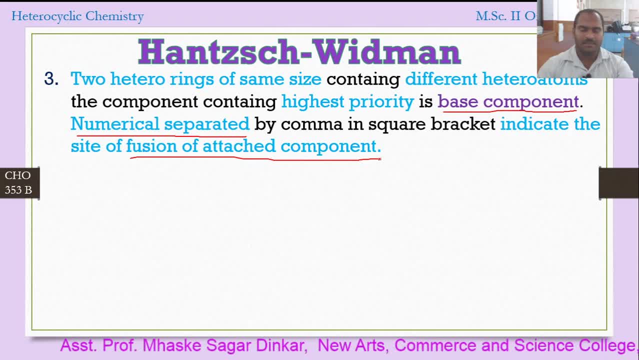 we can have a numbering. So let us illustrate this with the help of an example. So let us go for the example. Now, you can see here, these are the two rings which are of the same size, which are of the same size, and if we make a fuse component from these, then in that case we have to find 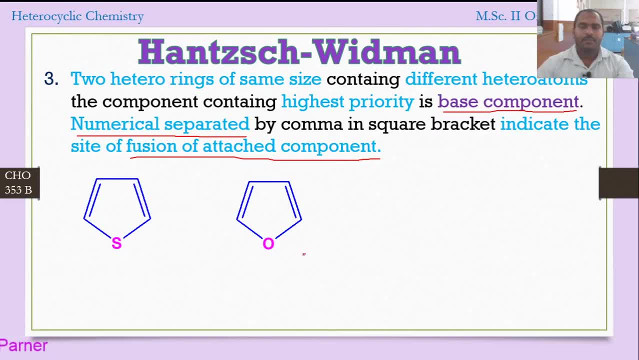 out, which is the base component. Now, here it is, a 5-member cyclic structure containing oxygen. here it is a 6-member cyclic structure containing sulfur. The two different heteroatoms are there: oxygen and sulfur. The highest priority is for the oxygen. therefore, this should be the base component. 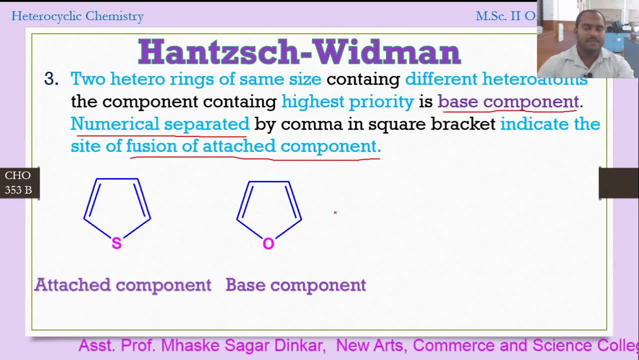 So it is the base component and this is the attached component. okay, So we are considering that furon is a base component and thiophene is an attached component. Now for base component. as we have already seen what will be the edges? Edges will be A, B, C and D. So we have to find out which is the base component and which is the attached component. Now for base component, as we have already seen what will be the edges: It will be A, B, C and D. 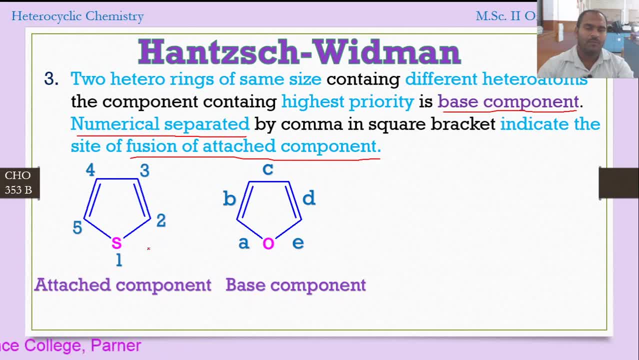 So we have to find out which is the base component and which is the attached component. And for attached component it will be 1, 2, 3, 4, 5.. There is a difference. A is denoted for this bond, B is denoted for this bond. C is denoted for this bond. 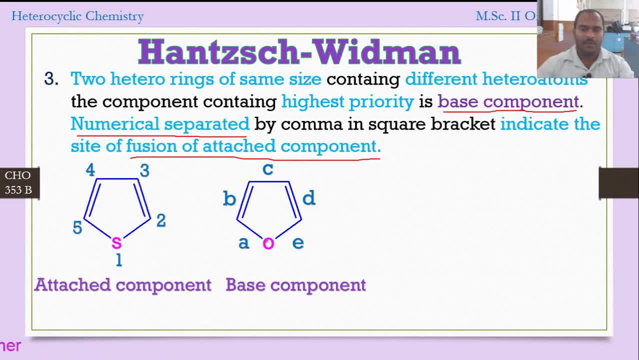 So here we are denoting the edges A, B, C, D, E for the base component, but for the attached component, what we are doing? we are giving the numbering 1,, 2,, 3,, 4 and 5 to the atoms. 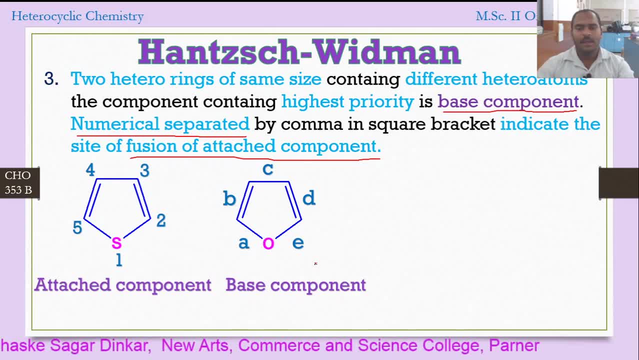 This attached component having the numbering to the atoms and base component having a letters to the bonds, that is, A, B, C, D, E and etc. Now, if these two combines and gives the formation of this fuel system, 5-5 fuel system. now, 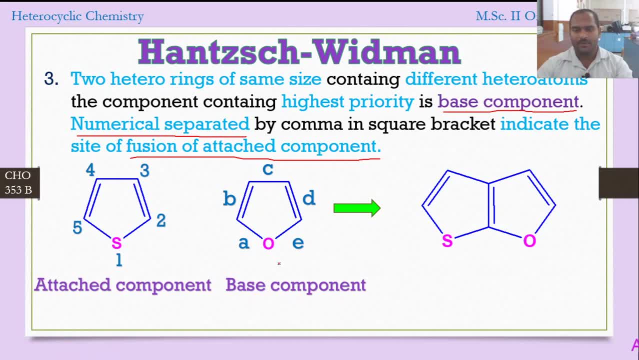 you can see here what will be the base component. base component is this: which containing the oxygen. Now, what should be the name of this? what should be the age? Age is A, B, so B's age is having a fuel system. now, this is B, and for this attached component, 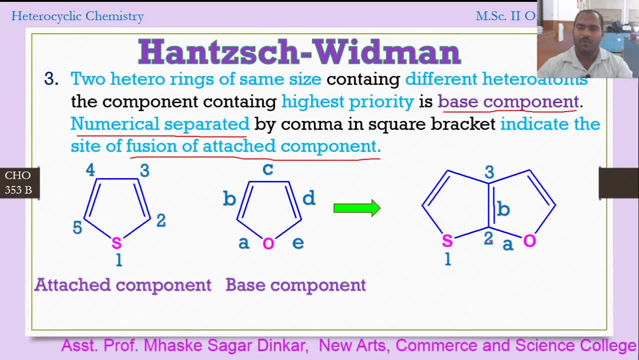 1, 2, 3, second and third atoms are involved in the fuse, so name will be thino right thiophene. so it is thino 2, 3, this 2, 3 what it indicates. it indicate atoms involved. 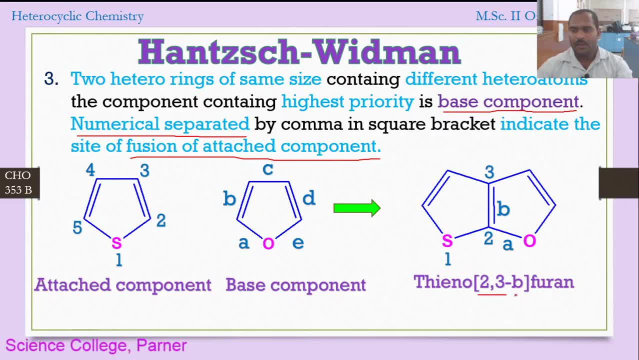 at the fuse position. from the attached component B We indicate site of attachment from the base component and furan is the name of the base component. ok, So now compound is having IUPAC name: thino square bracket 2, 3 dash B square bracket. 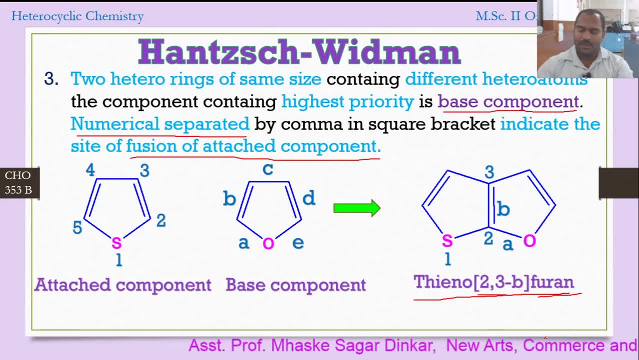 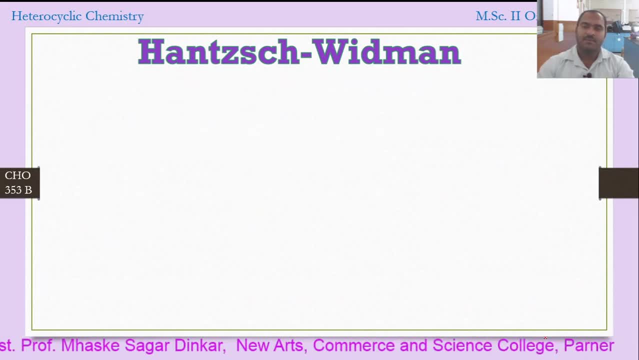 complete furan is the name of the compound. ok, So that much is the symbol for the heterocyclic building with the same size. Now let us consider further. for the next, In case of an unequal size, largest ring is considered as a base component. Previous case it was equal. now, in case of an unequal size rings, here we are considering that the largest ring is considered as a base component, but remember that largest ring also should contain the heteroatom. ok, So that largest ring is considered as a base component. 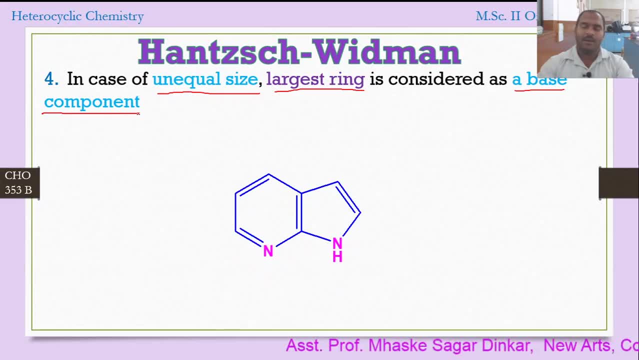 Now here we can see the example Directly. we have taken the fuse system. Now here there are 2 cyclic system. one is a 6 member, other is a 5 member. ok, 6 member is a largest. therefore, this is the base component, while the other is a attached. 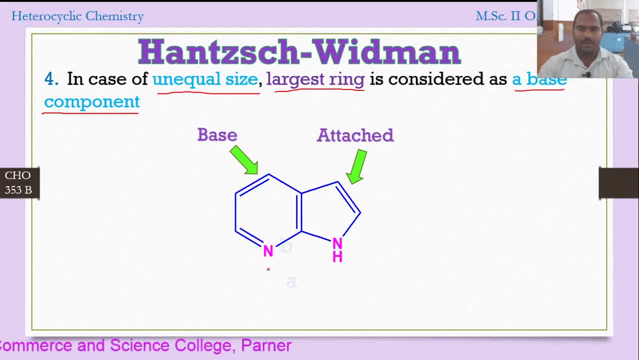 component. ok, Now, similar way we have to go for the identification of the edges, and the number, that is, the B edge, is attached for the fuse system, and here we are having numbering 1,, 2, 3.. So what will be the name? 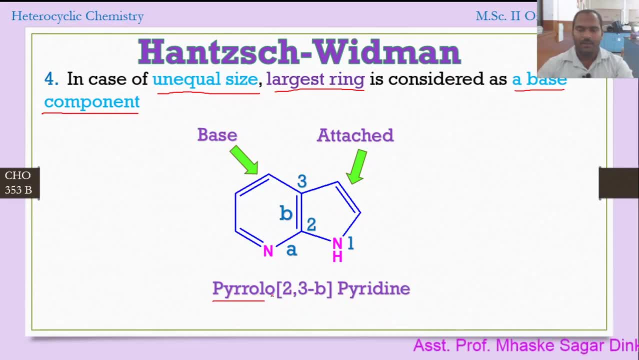 Pyrello right, Pyrello 5. member. therefore Pyrello 2, 3, these are the edges and B is the edge from the base component and pyridine is the name of the compound. So base component, therefore name of the compound will be Pyrello square, bracket 2,. 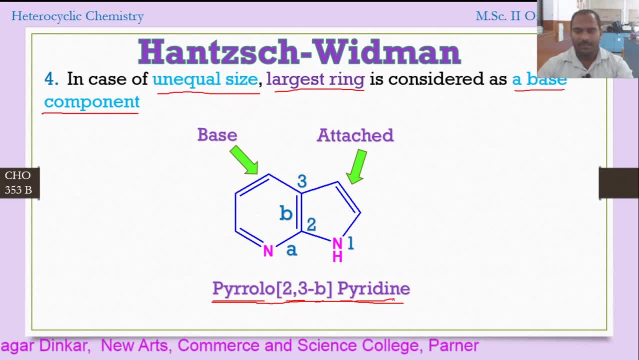 3: B square bracket: Ok. B square bracket- complete pyridine is the name of the compound, ok, or iPad name of the compound. So in case of an unequal size, largest ring is a base component. here you can see it is. 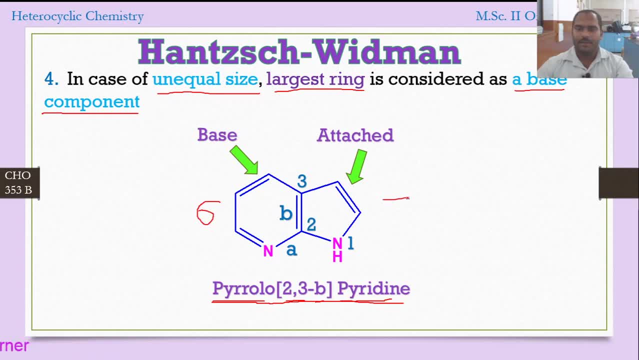 a 6 member, therefore it is a base component. it is a 5 member, therefore it is a attached component. Both are having the heteroatom, but the system with the 6 atoms is considered as a base, while 5 atom is considered as a attached system. 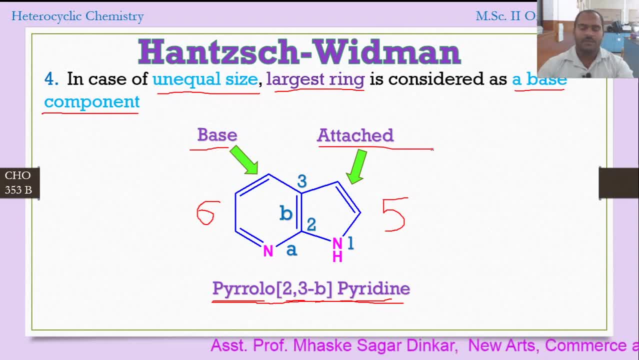 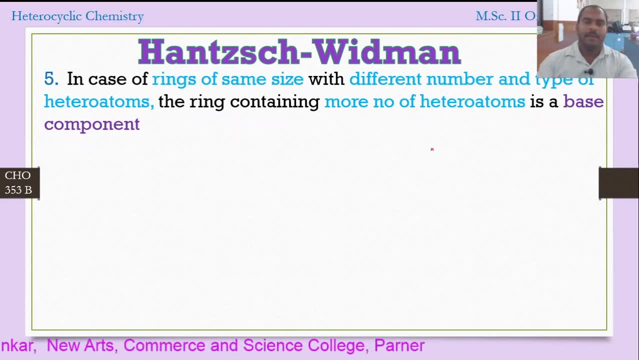 Ok, So this is the rule number 4.. Now we will go for the next. In case of a ring of same size with different number and types of heteroatoms that we are considering, the ring that contains more number of heteroatoms is a base component. 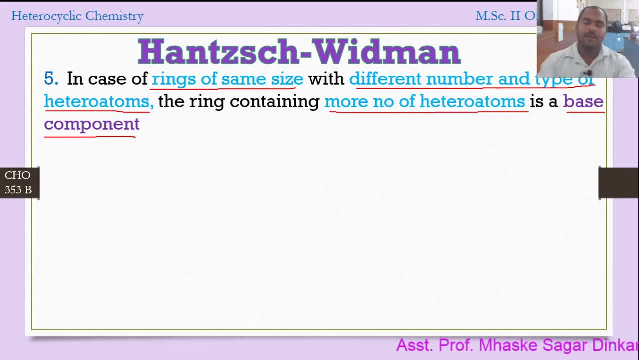 So when we are considering a ring of a same size with different number and types of heteroatoms, the ring contains more number of heteroatoms in a base component. Ok, So let's consider the example for illustration Now. here you can consider: this is the 5 member ring. this is also 5 member ring. 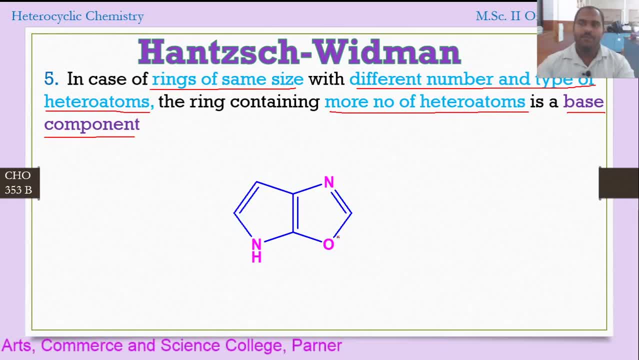 Ok, both are of the same size, but they are having the different number and types of the heteroatoms. This contains only nitrogen. this has nitrogen and oxygen. So here we are having the different type of the heteroatoms and different number of. 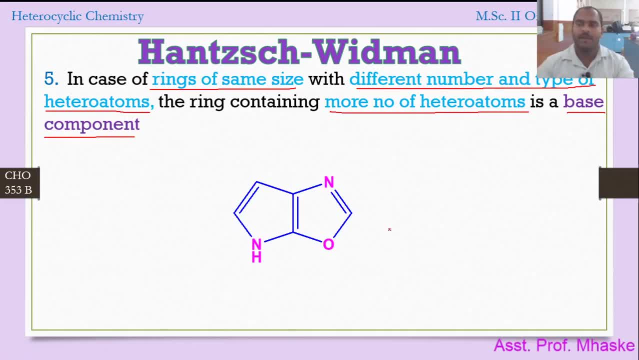 the heteroatoms. So the ring containing more number of heteroatoms is a base component. So this is the base component where we are having a 2 heteroatoms. So out of these two, this is the base component and this is the attached component. 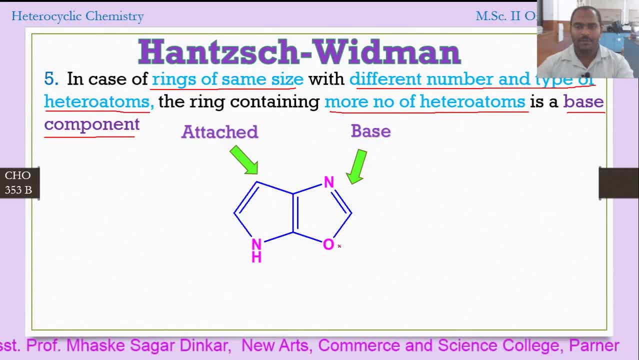 Size of the ring is the same, But there are 2 heteroatoms. Therefore, this is the base component and this one is the attached component, Even though the size is same and there are different heteroatoms. So again we are having the ages. 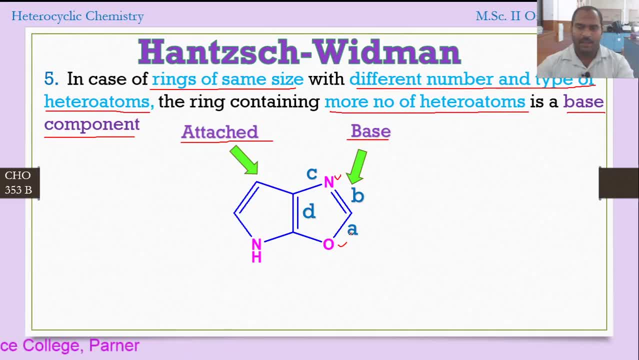 But now here there is a different age. Why A, B, C and D? Why not from this side? A B C? Because there should be the least distance between the 2 heteroatoms. Ok, So oxygen and nitrogen- here is only one carbon in between them. 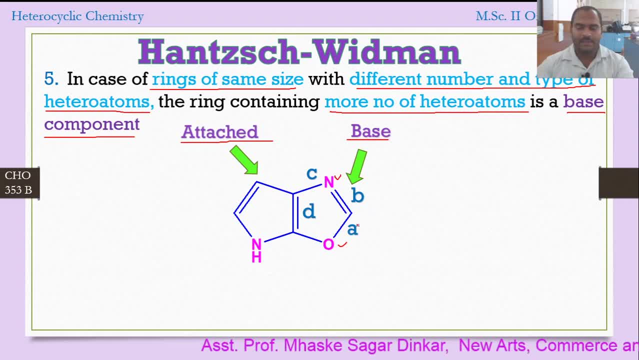 Here are 2 carbon. Therefore, the ages number, or ages later, will start from this side: A, B, C, D. Ok, Now for this other side. it is simple: First to the nitrogen, second to this carbon and third to this carbon. 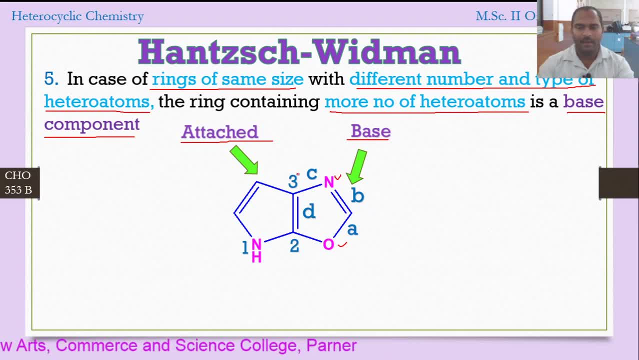 Ok, So in square bracket now we are having 2,, 3 and D. So what will be the name? Pyrello? Why pyrello? Because it is a 5-member attached component with the nitrogen. So pyrol is the component base attached component. 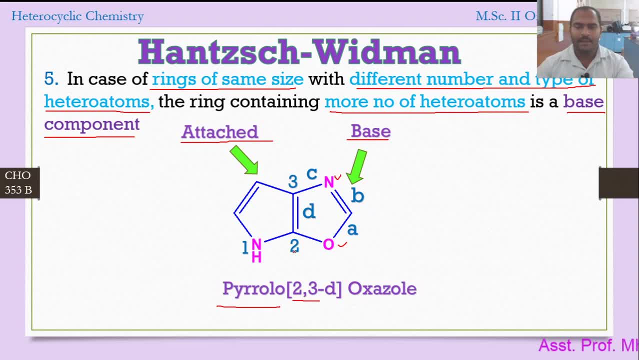 Therefore it is the pyrello. 2, 3 indicate a site of attachment for the attached component And D indicate the age of attachment of the base component And oxazole that will be the base component, So compound name will be pyrello. 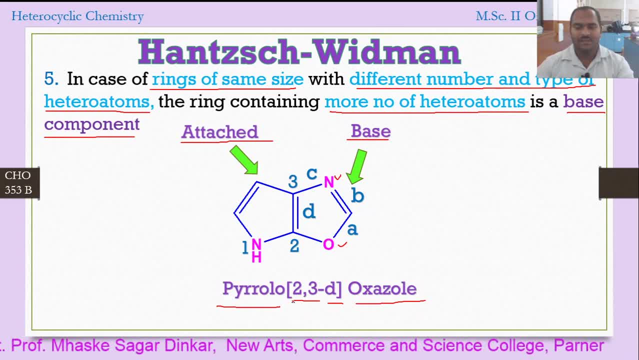 Square bracket 2, 3.. D square bracket, complete Oxazole will be the name of the compound or I bag name of the compound. So in case of a same size ring and with a different heteroatom and different number of heteroatom, the base component is the component where there are the more heteroatoms are present. 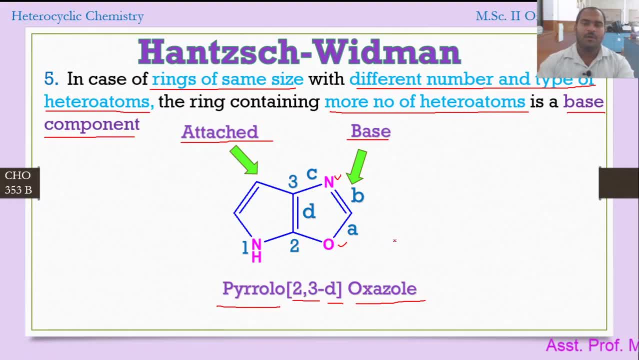 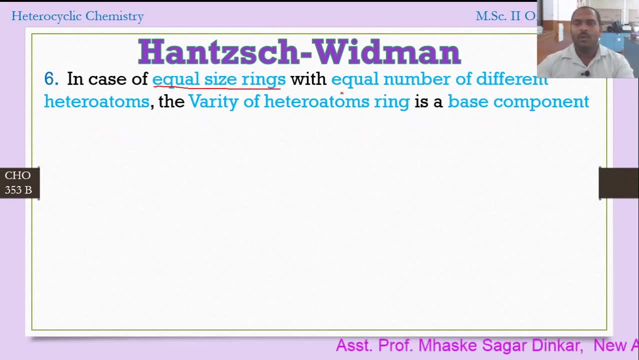 Ok, So that we are considered. Now let us go for the next rule. In case of an equal size ring with Equal number of different heteroatoms, Equal number of different heteroatoms. The variety of a heteroatom ring is a base component. 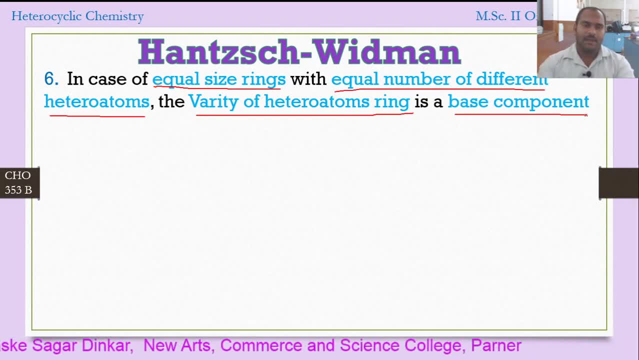 So here, what is considered? Here it is considered that, in case of an equal size ring in an equal number of a different heteroatoms, The ring which is having a variety of a heteroatom ring or variety of heteroatom in the ring. 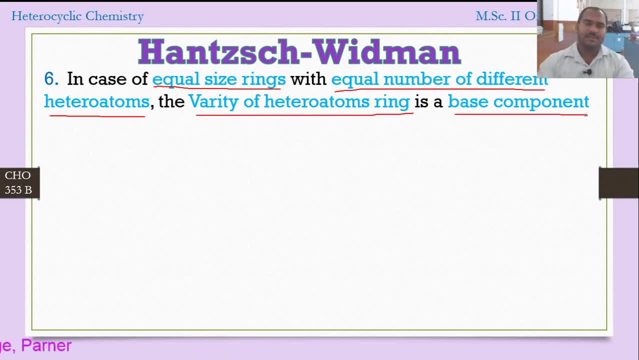 That ring is considered as a base component. Now let us consider the example Now. here you can see: Ring is of an same size, The number of an heteroatoms are same, But they are different type of the heteroatom. 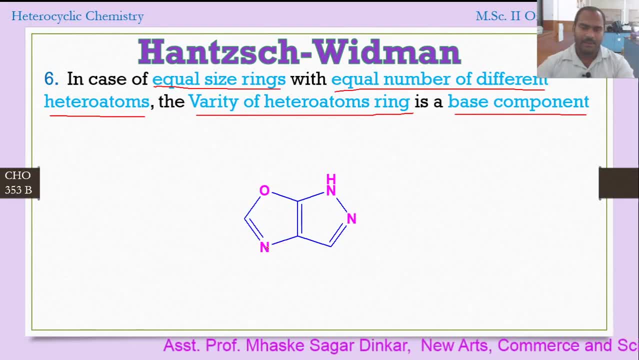 Here we are having the two nitrogen atoms, while here we are having nitrogen and oxygen. Ok, So what we are having? I remember cyclic structure, Both I remember. therefore, equal size rings are there. They are having equal number of an heteroatom. 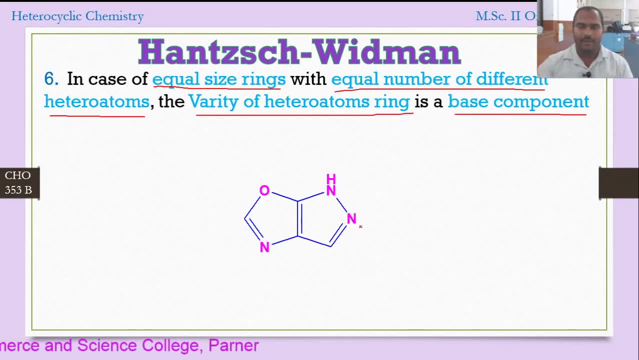 That is a two, two heteroatoms, But in one ring there is only nitrogen present as heteroatom, While in second ring, oxygen and nitrogen are present as a heteroatom. So according to this rule, The ring which is having a variety of heteroatom, that is a base component. 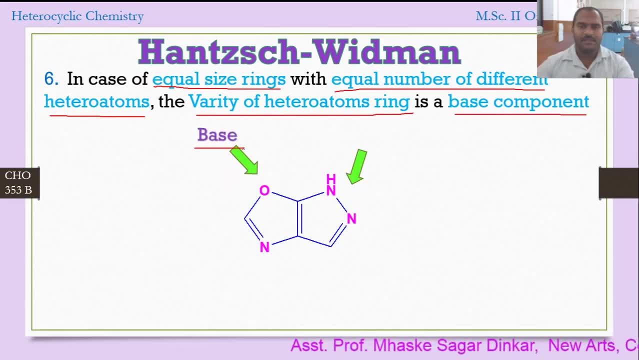 So which will be the base component? This side will be the base component which containing oxygen and nitrogen as a variety, While other side is attached component. Why attached component? Because in this case we are having the same heteroatom Variety is more for this side. 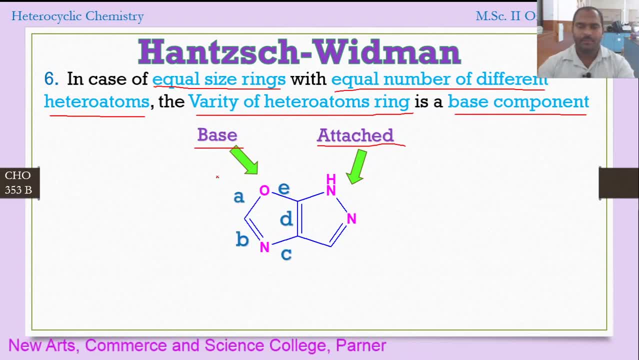 Therefore it is a base. So what will be the age here? A, B, C, D and E? Out of that, D is the age which is attached for the base component. And here, if we give, Here if we give the number, 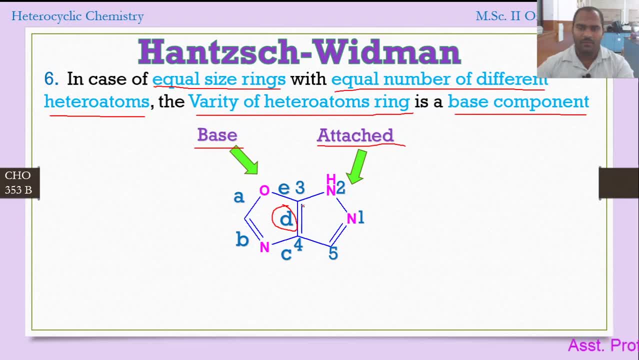 Number will be 1,, 2,, 3 and 4.. So 3 and 4.. These are the atoms which are present at the fused position. So name will be 1H- 1H-Pyrazole-4,3-D-Oxazole. 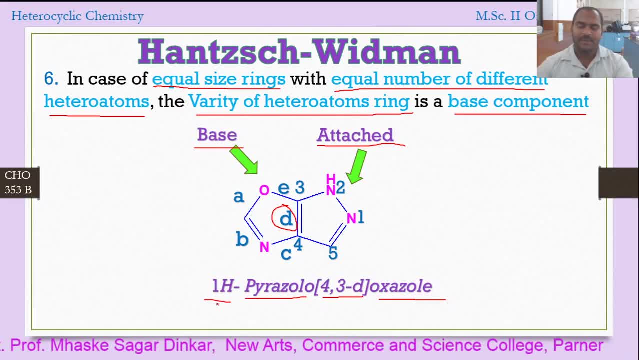 Okay, that will be the name. Now let us consider the explanation of this name. 1H. Now here, nitrogen. There should be the H, But due to presence of a double bond, there is an abscess. Therefore 1H, which is written in the form of an italic. 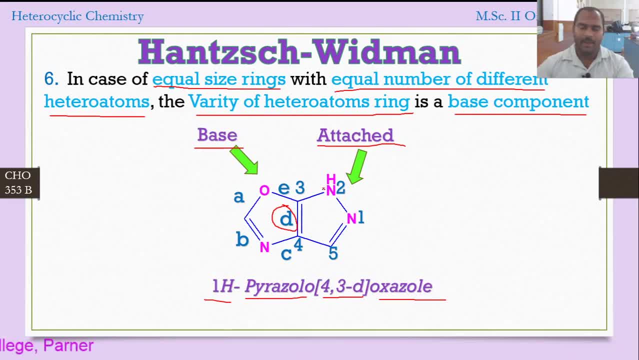 Pyrazole. Pyrazole. Pyrazole is the name of the parent, So here we are having a replacement of a large E by O, So Pyrazole in bracket square, bracket 4, 3.. 4, 3.. 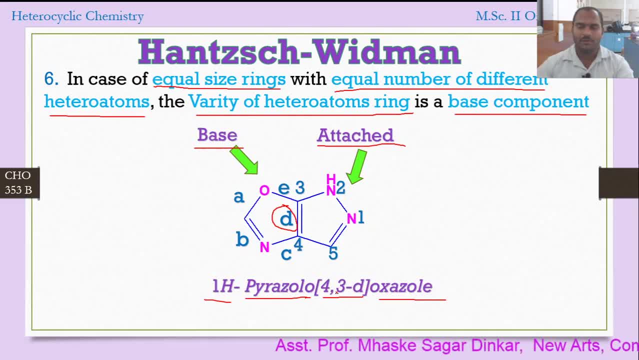 It will indicate the position. Here we can mention 3,, 4, also Dash D. D is the H from base component. And what is the base component? It is a oxazole, So name of the compound will be 1H-Pyrazole, square bracket 4, 3-D-Oxazole. 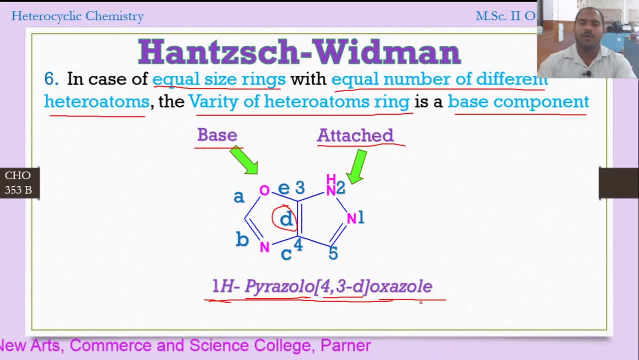 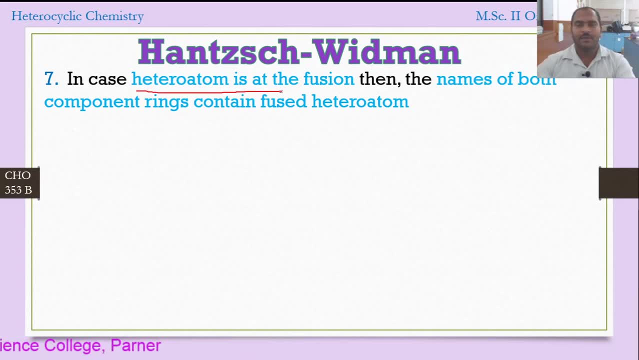 That will be the name. Okay, Now let us go for the next room. In case of a heteroatom is at the fusion. It is one of the interesting case, Then the names of both component rings contain the fuse heteroatom. 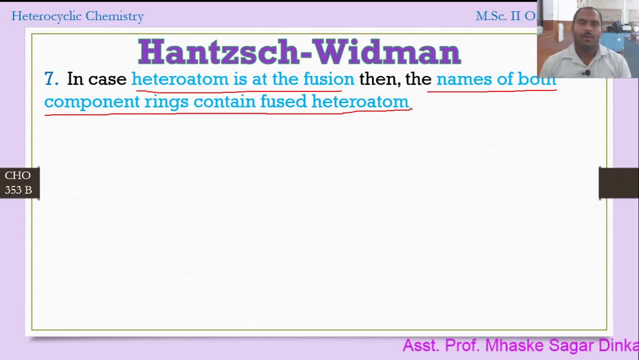 That we have to consider. So, when there is a heteroatom is present at the fusion, In that case, what we have to consider, We have to consider that that heteroatom is attached to the both component, The base component as well as the attached component, or it is belonging from the both. 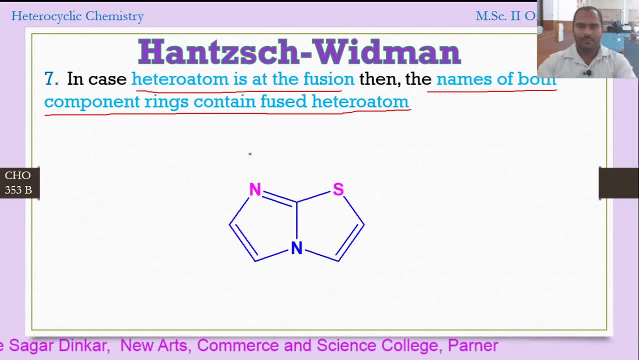 the rings. So let us consider the example Now. here You can see Both are 5 member ring, One having nitrogen, other having sulphur, and this nitrogen, the nitrogen which is shown in the blue colour, it is in the fuse position. 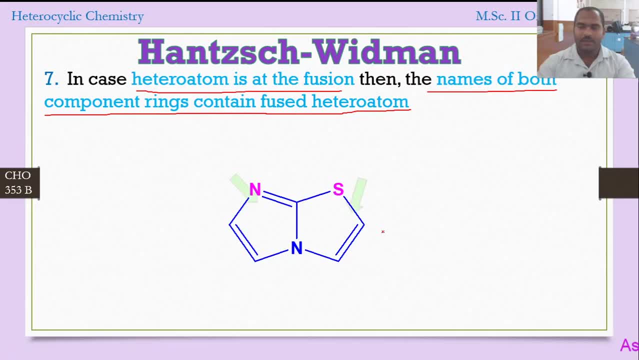 Okay, So for this, what we have to consider, What is the base component? Base component obviously will be this side, because it is having a variant sulphur and nitrogen, While here is the nitrogen nitrogen. So this is the base component. 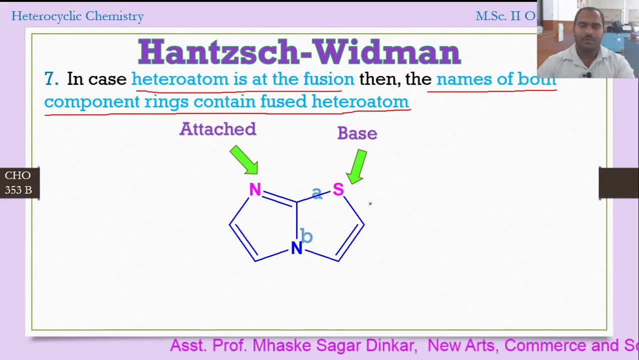 This is the attached component. So what is the H? H is a, B, where we are having an attachment on the base side, and what will be the number? It will be 1,, 2, 3.. 1, 2, 3.. 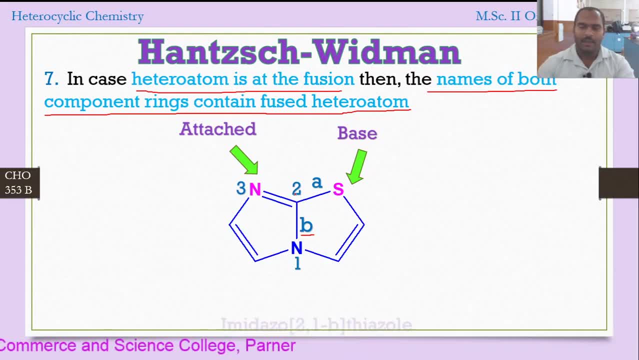 So here we are having 1 and 2.. That is the attachment. So here we are having the name imidazo: 1, 2 or 2, 1.. B is the attachment. So here we are having the name imidazo. 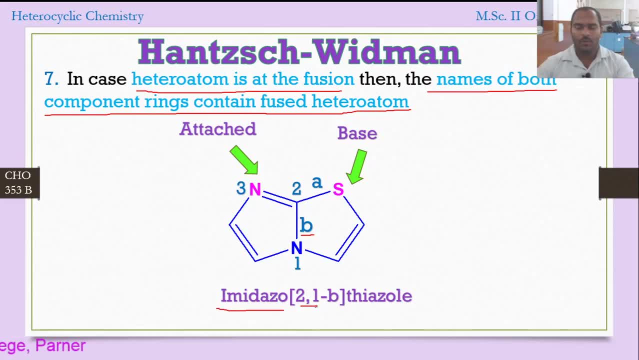 So 1, 2, or 2, 1.. B is the attachment, So we have to consider b is the age and thiazole is the name of the compound. so imidazole 2: 1 is square bracket 2: 1. 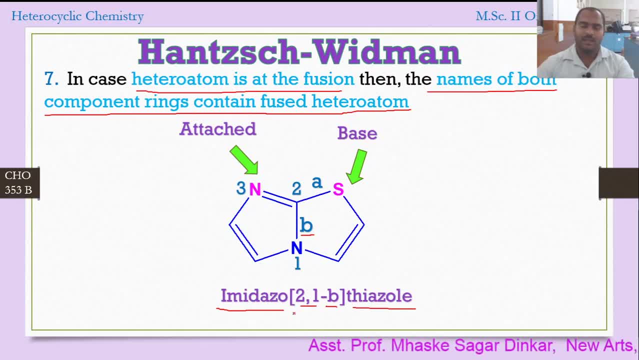 dash b, square bracket. complete thiazole is the name of the compound. so here at the fuse position there is a nitrogen. so nitrogen we are considering with the both, so imidazole with the base attached component and thiazole with the base component. so this nitrogen is considered for. 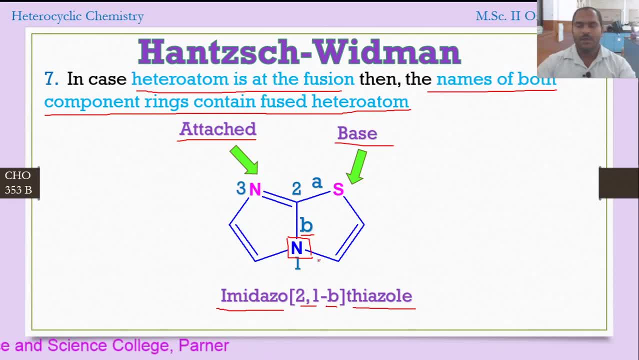 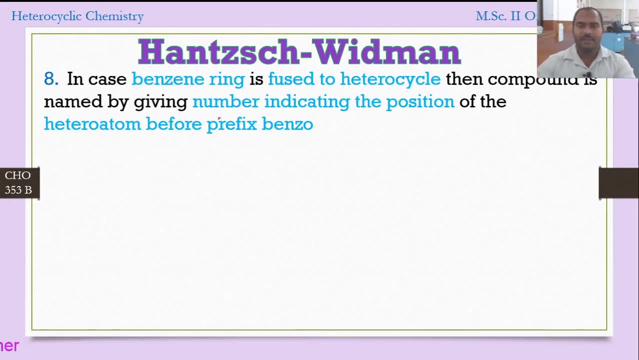 the both base and the attached component, that is, a fuse nitrogen. okay, now let's go for the next rule. in case of an benzene ring is fused to the hetero cycle. in case of a benzene ring fused to the hetero cycle, then the compounds is named by giving. 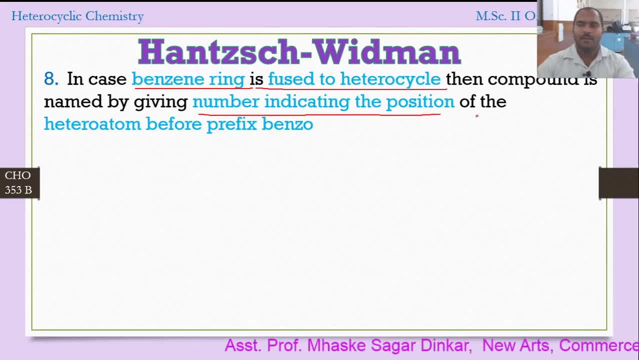 the number indicating the position of the hetero atom before the prefix benzo. so what we are doing, we are doing, in this case, the numbering which indicates the position of a hetero atom before the prefix benzo. so when benzene is attached with a fused heterocyclic system, in that case we are. 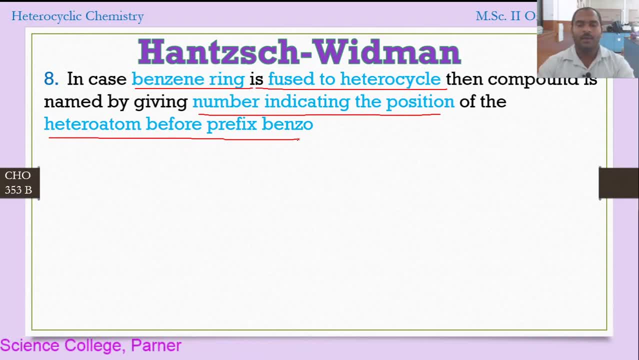 having the number which indicate the position of the hetero atom. so here we are considering the example. now you can see here: this is the benzo component which is attached to the hetero atom, or cyclic ring or heterocyclic. so what should be the name or what should be the number? number should be given in a 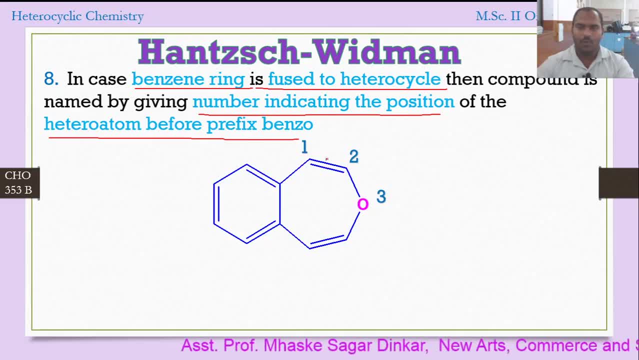 such way that it should have the smallest number to the hetero atom: 1, 2, 3. okay, if we go this direction is one and the same, so name of the compound will be 3-benzo-oxy-epene. right, that will be the name. 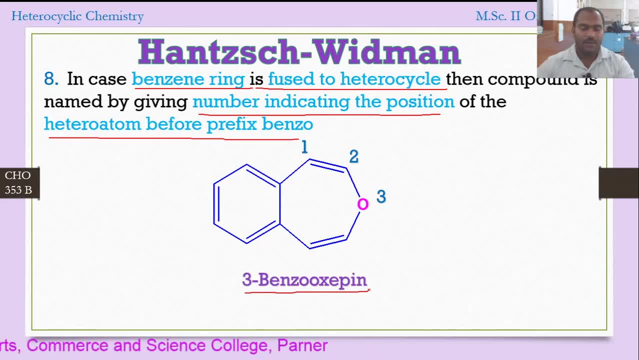 of the compound, without known the name, does enter air where we are having amazing attachment. what is indicate? 3 indicate the position of an oxygen. benzo is attached component and oxyepine is the heterocyclic ring which attaches to the benzene is the seven member cyclic structure having oxygen and therefore it is oxy epine. therefore, 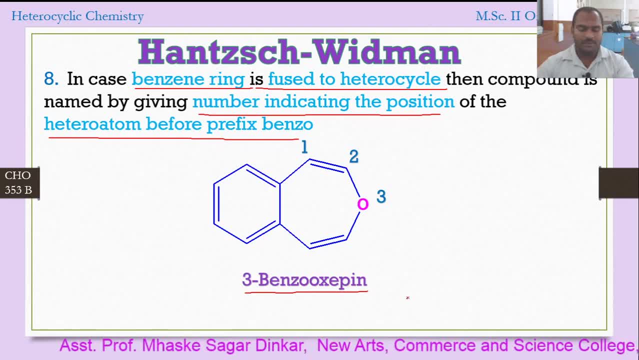 The name of the compound is 3-benzo-oxy-EV. So these are the rules for the nomenclature of the fused heterocyclic system with the help of a Hans-Willemann system. So these 8 rules are helpful in giving the IUPAC nomenclature for the heterocyclic compounds which are having a heteroatom with the fused heterocyclic system.